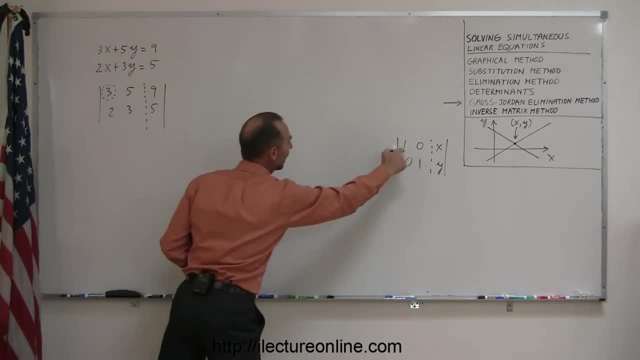 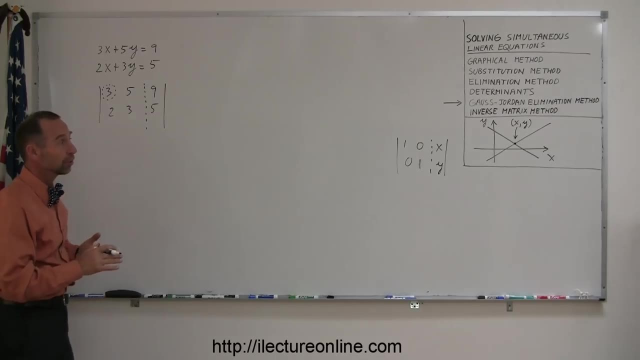 and the first thing you want to do is turn this three into a 1, and you can do that by simply taking the whole first row and divide the whole row by 3.. And remember, whenever you use the Gauss-Jordan elimination method, you must do exactly the same thing to everything in the same row. 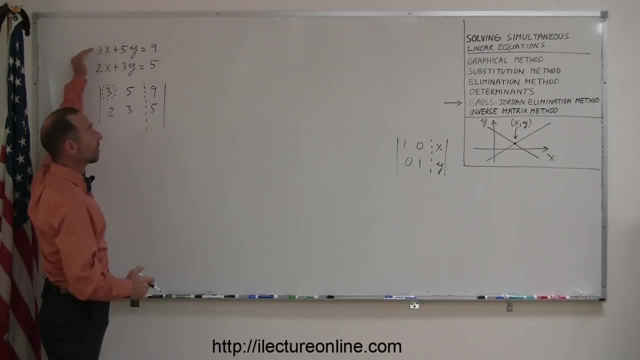 which means you must do the exact thing in everything in the same equation, or do the same thing in both sides of the equation. So we're going to take the first row and replace it by 1 third, the first row. That's the same thing as saying I'm going to take the first row and divide it by 3.. 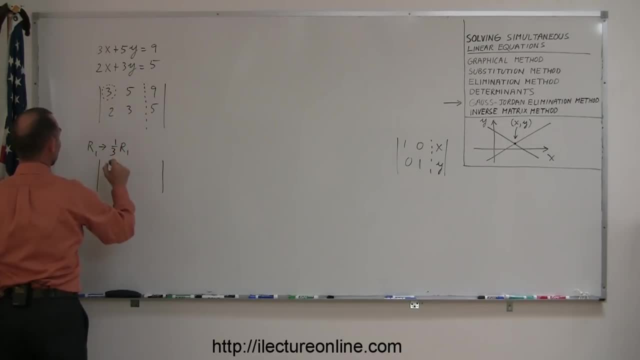 When you do that, you get the following: You get: 3 divided by 3 is 1,, 5 divided by 3 is 5 over 3,, 9 divided by 3 is 3, and the second row goes unchanged. 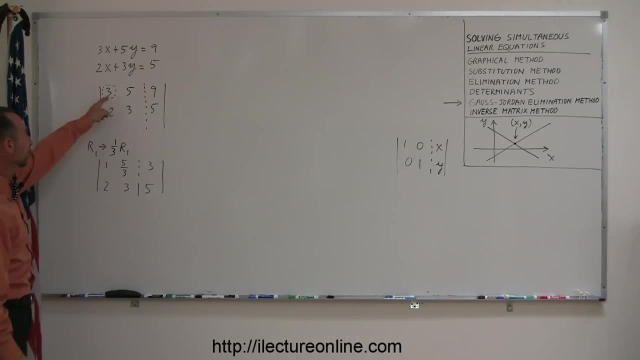 All right, we're partway there. We have now taken our first number right here and turned it into a 1 to make it look like this. The second thing we want to do is take this number right here and turn it into a 0.. 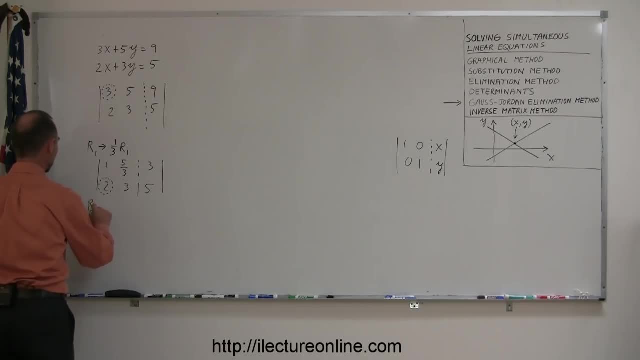 How do we do that? Well, the methodology says that we take the second row and replace it by the third row. So we're going to multiply the negative of this number, times the row with the 1 in it and adding it to the row that we're trying to change. 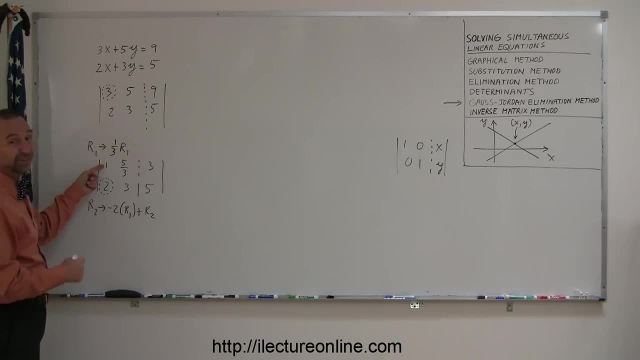 So we're going to multiply this by negative 2, which gives us a negative 2, add it to the 2 to turn it into a 0. Okay, if we do that, we get the following: Now notice, we're not changing the first row at all, so we can rewrite that. 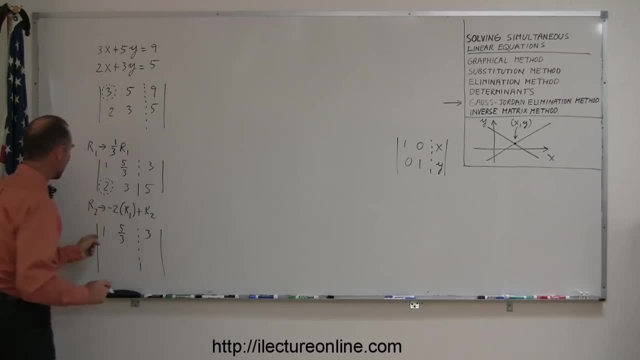 1, 5 over 3, and 3.. Multiplying this 1 by a negative 2, that gives us negative 2.. Negative 2 added to 2 gives me 0.. Multiplying this by a negative 2, so negative 2 times r1, means negative 2 times this. 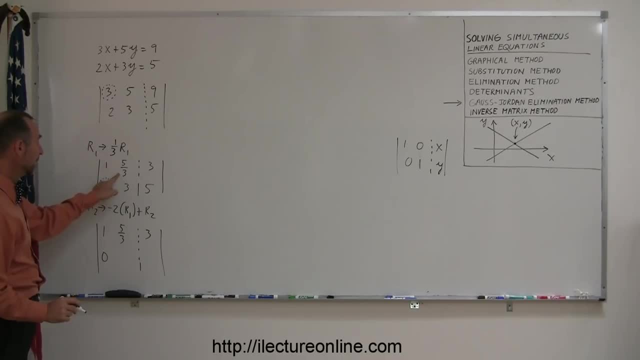 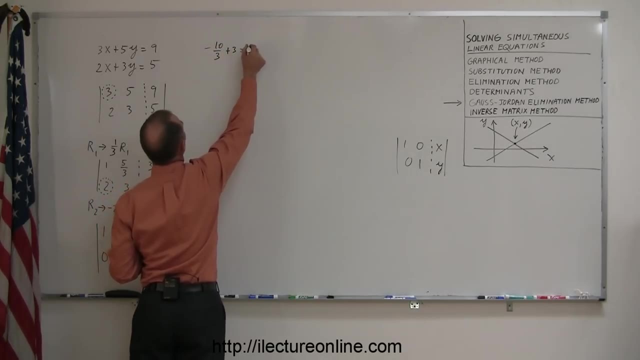 Negative 2 times. this gives me a negative 10 over 3, and I add that to 3.. Now let's do that on the side We have. negative 10 over 3 added to 3 is the same as negative 10 over 3, adding it to 9 over 3,. 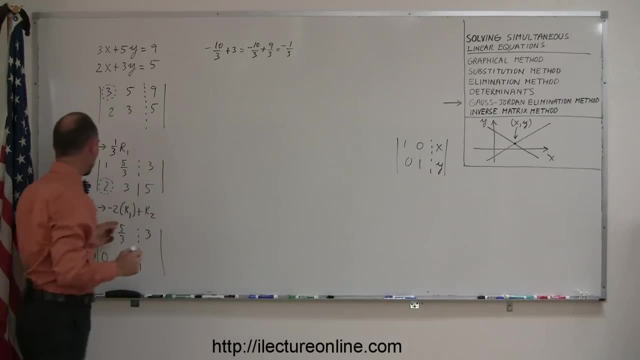 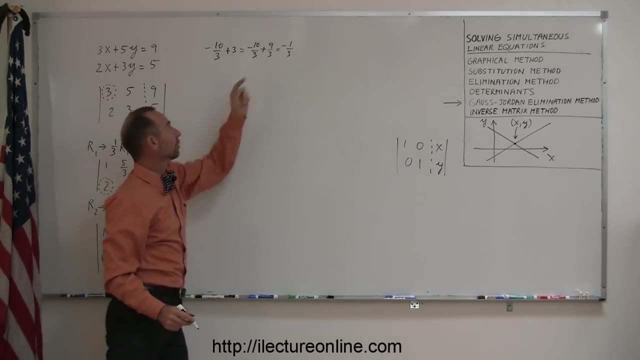 which is minus 1 over 3.. So if I multiply this by negative 2, I get negative 10 over 3.. I add it to 3, I will get negative 1 over 3, and I put that down in here. 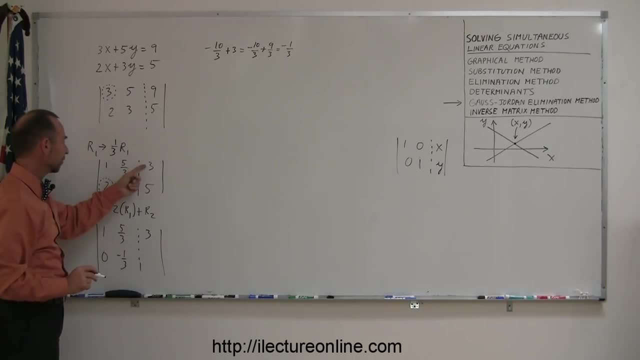 Over here. I'm multiplying the 3 by negative 2, that gives me negative 6, add it to 5, that gives me a negative 1.. All right, halfway there I get the 3 and the 2 now changed to 1 and a 0,, which is exactly what I want. 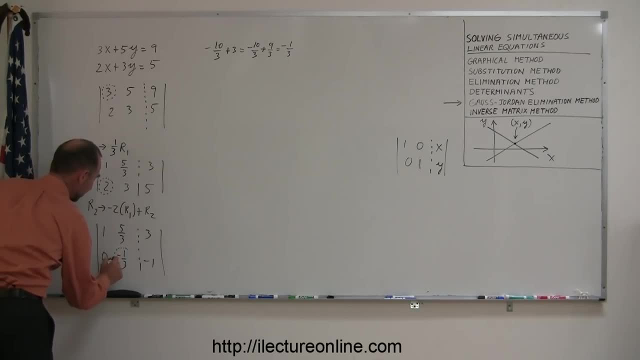 So next I work on this number right here I go to the second column and I go to the number where I want to change it to a 1. To do that I need to take this number and multiply it times a negative 3.. 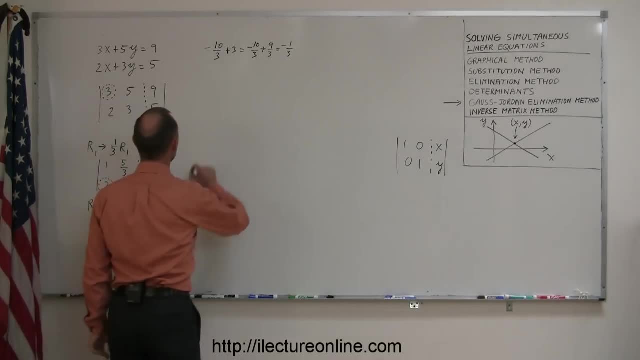 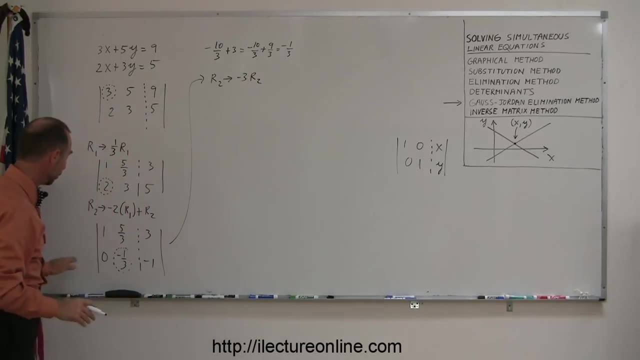 If I multiply this by negative 3, I get 1.. So that means I'm going to take my second row and replace it by negative 3 times the second row. Simply said, I'm taking the whole second row and multiplying every number in the second row by negative 3.. 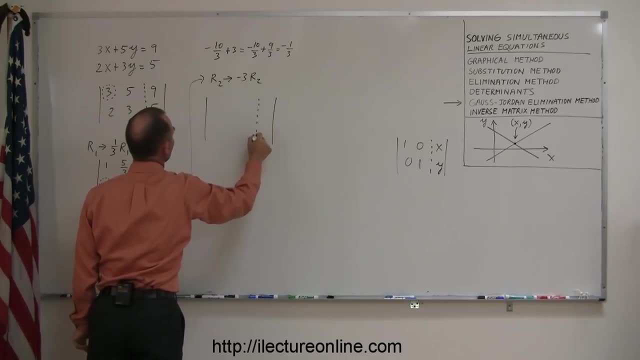 When I do that, I get the following: Notice that nothing changes in the first row, so that still remains as a negative 3.. Notice that there's a 1,, a 5 over 3, and a 3. The 0 doesn't change. 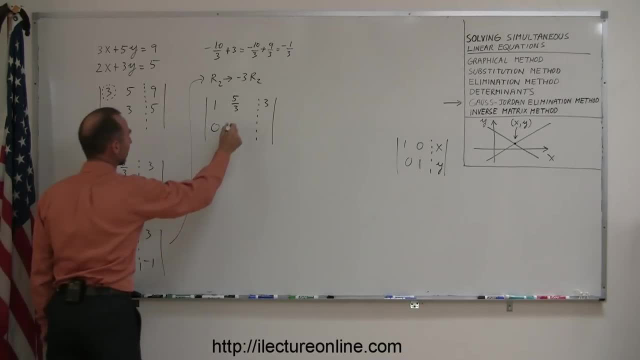 If I multiply this by a negative 3,, I get a 1.. If I multiply this by a negative 3,, I get a 3.. Almost there, Notice. I have a 1,, a 0, and a 1,. just what I need over here. 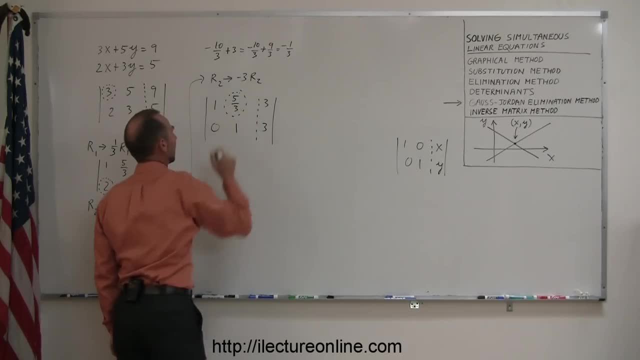 Now I'm going to need to take this number and turn it into a 0. And using the Gauss-Jordan elimination method, the rule is that you take the first row, the row you want to change the number to, and replace it by the negative of this number, which is minus 5 over 3,. 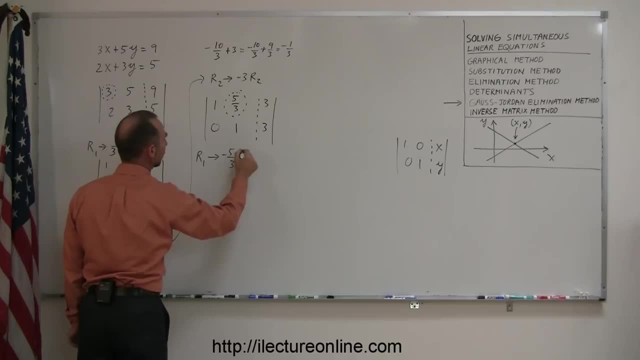 multiply it, times the row that has the 1 in it, which in this case is R2, and add it to the row that you're changing, which is R1.. So simply said: take this number, multiply it by negative 5 over 3,. 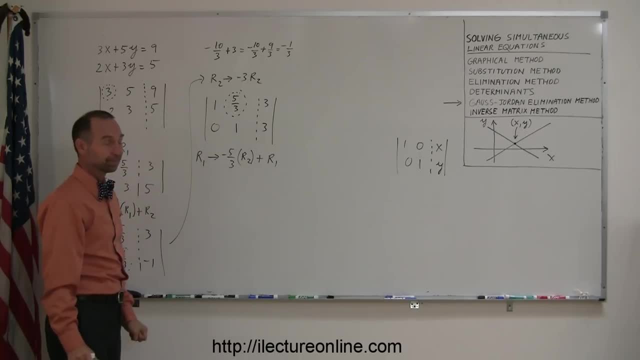 and add it to that number and it'll turn into a 0.. If we do that, what do we get? Well, first of all, the second row does not change: 0,, 1, and 3.. In the first row, this is already a 1. that will not change. 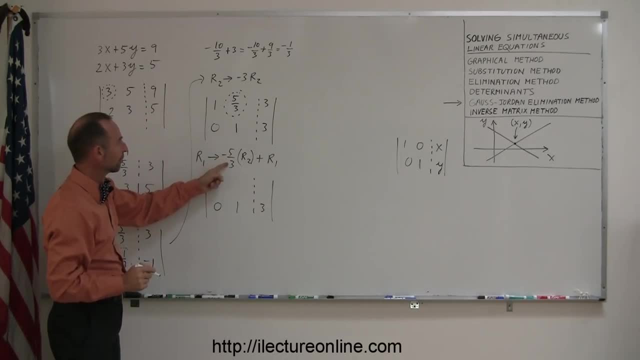 Now, taking this number, multiply it by negative 5 over 3, times that number, that's negative 5 over 3, add it to positive 5 over 3, gives me a 0.. Taking this number, multiply it, times the negative 5 over 3,. 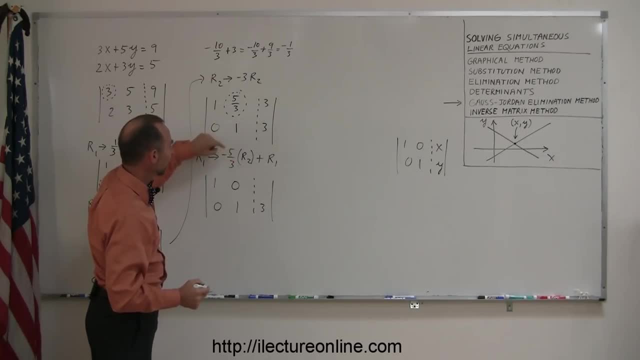 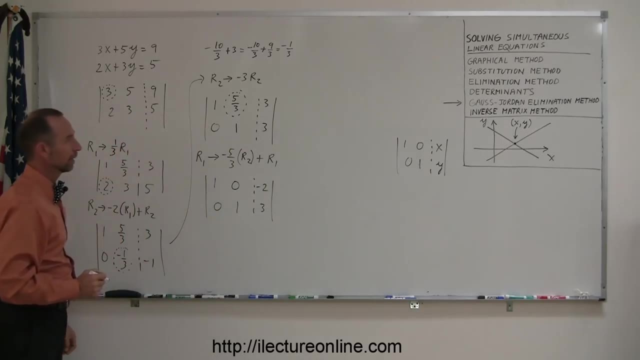 notice, if I multiply this times this, the 3's cancel out and end up with negative 5,. add it to a positive 3, and end up with a negative 2.. And now I'm done, because I have the exact values for x and y. 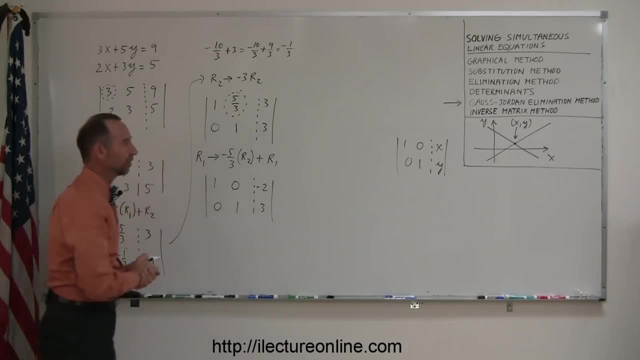 I have 1, 1, and 0, 0 on the left side, so that's how I know I'm done, and I can then say that x equals negative 2, and y equals positive 3.. And just to make sure we did it correctly, let's plug those values back in the original equations. 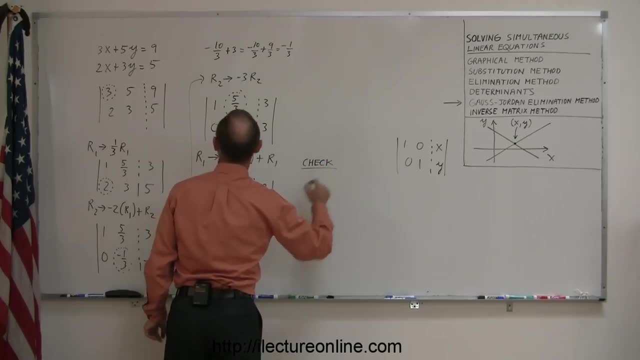 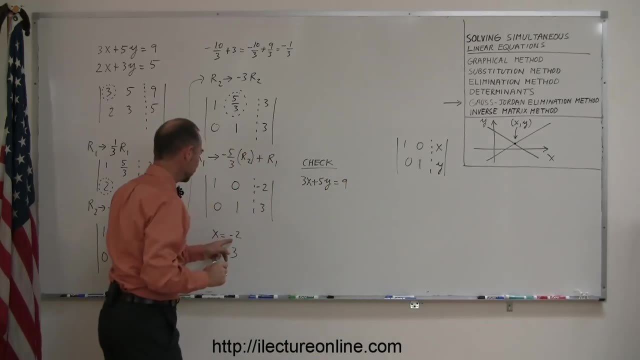 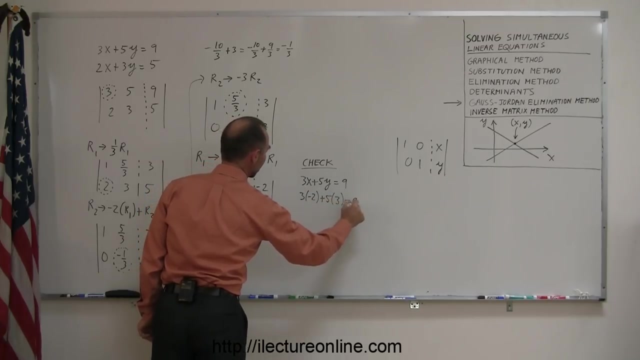 so we're going to check: 3x plus 5y equals 9,. plug in negative 2 for x and a positive 3 for y, so 3 times negative 2, plus 5 times 3, is that indeed equal to 9,? so negative 6 plus 15,. 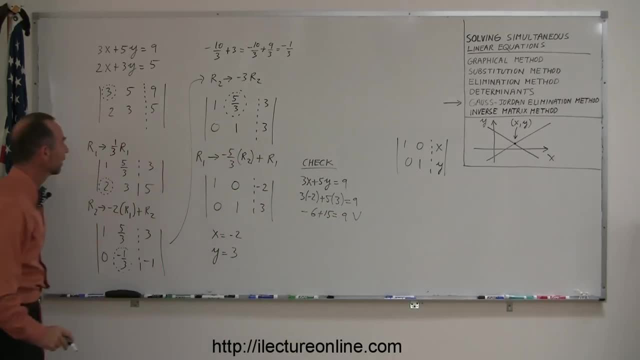 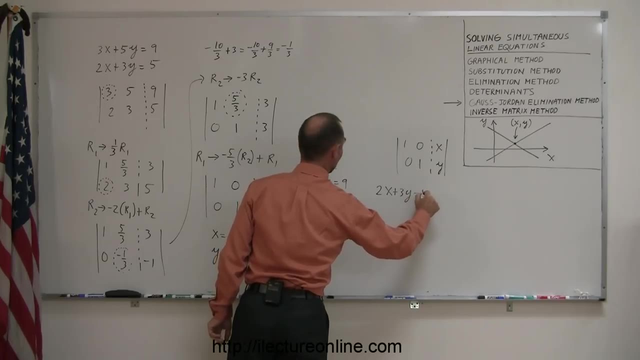 yes, indeed, that's 9, so that's correct. and one more check, taking the second equation, so we have 2x plus 3y equals 5, again plugging in the negative 2 and 3 for x and y. 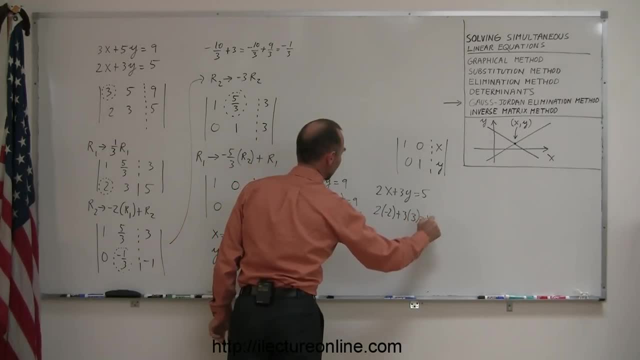 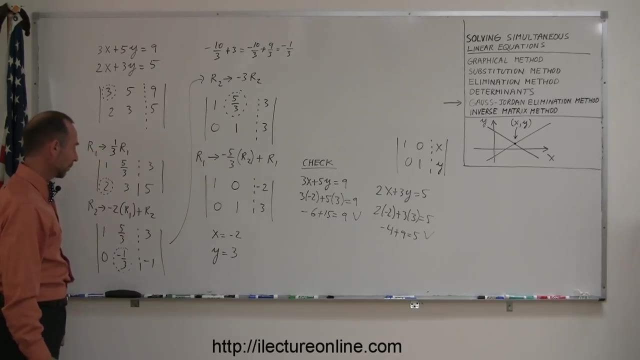 we get 2 times negative: 2 plus 3 times 3 equals 5, or negative: 4 plus 9 equals 9, yes, indeed, that's equal to 5, so we just saw that we did it correctly, and those are the. 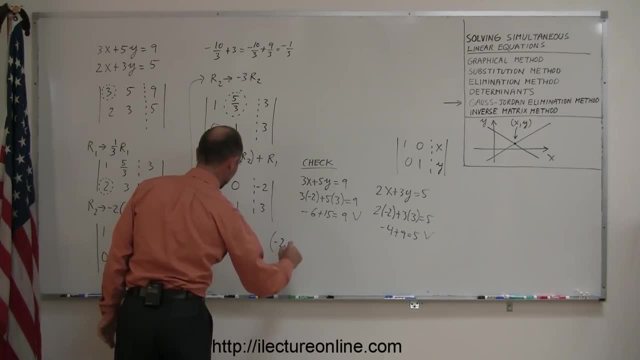 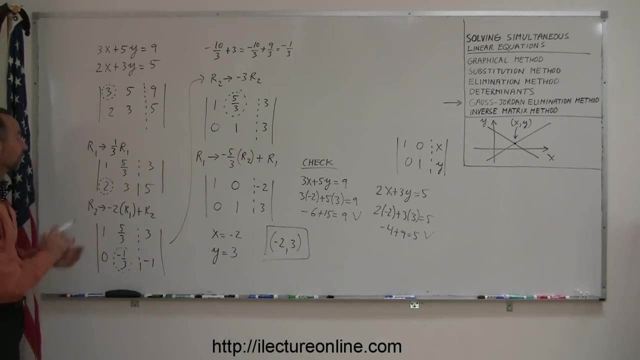 x and y coordinates. you can also write it like this: x equals negative 2, y equals 3, there's my solution to those two equations. that's the point where the two equations cross.